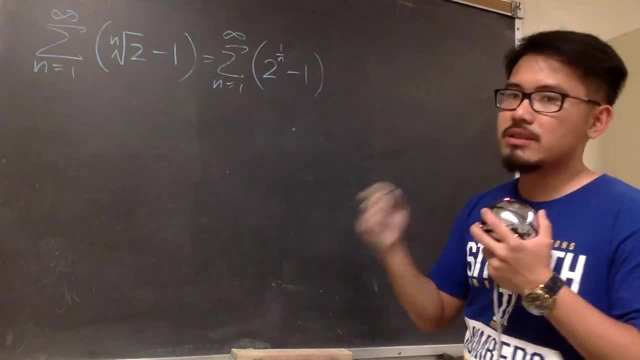 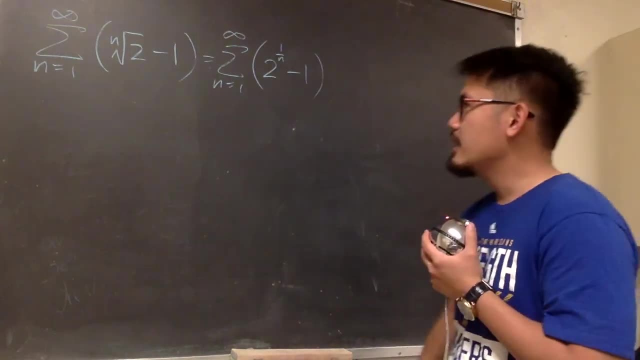 2 to the 0th, power is 1.. 1 minus 1 is 0.. Unfortunately, tests for divergence doesn't work because we do end up with 0. So we are going to do some tests for divergence. So now what? 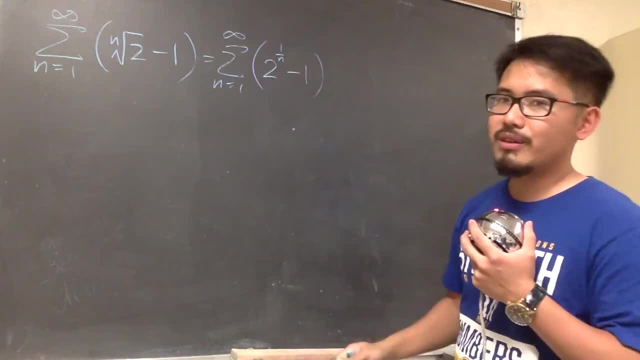 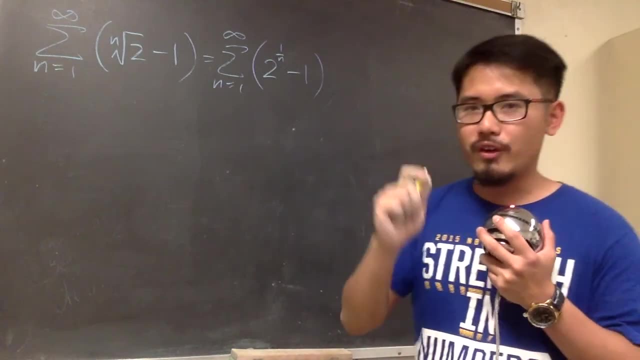 Well, after we change the nth root to 1 over nth power, this is kind of suspicious Because if you look at sigma, n goes from 1 to infinity, 1 over n. That's the harmonic series and that diverges right. 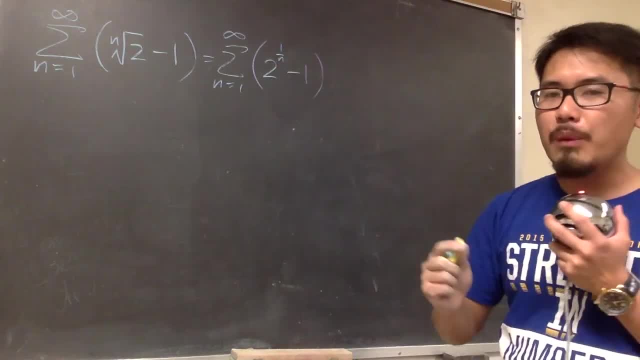 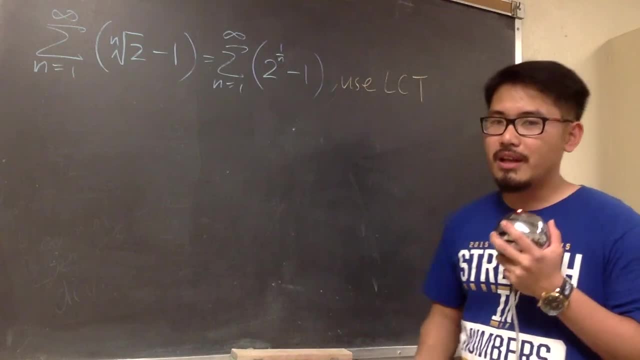 So maybe I can do some comparison with this And I would like to use the limit comparison test for that to see if we can draw any conclusion, And I would like to tell you if you want to use the direct comparison test. unfortunately, in this case it wouldn't work. 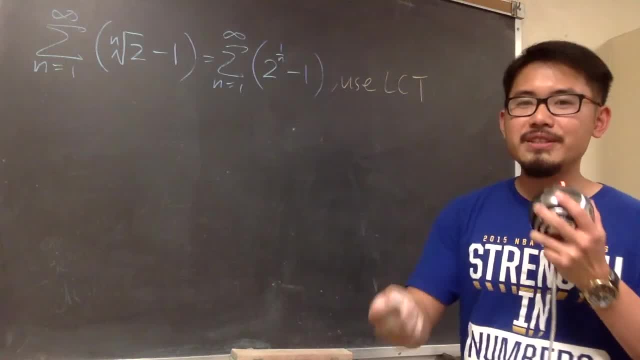 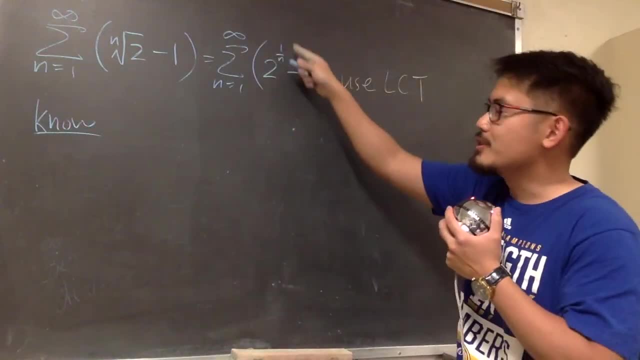 Limit comparison test is the way to go, But I'm just going to try it and convince you that it will work. So let's put down the things that we know, which is the, you know, just the 1 over n. 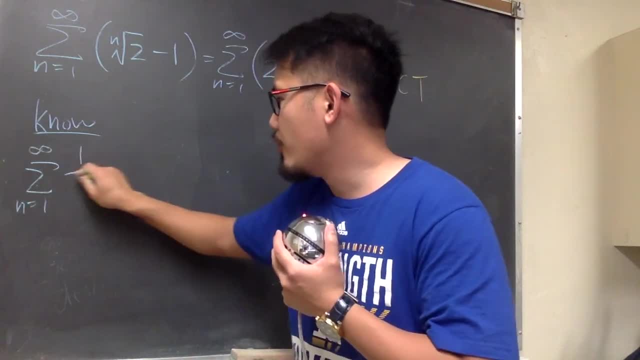 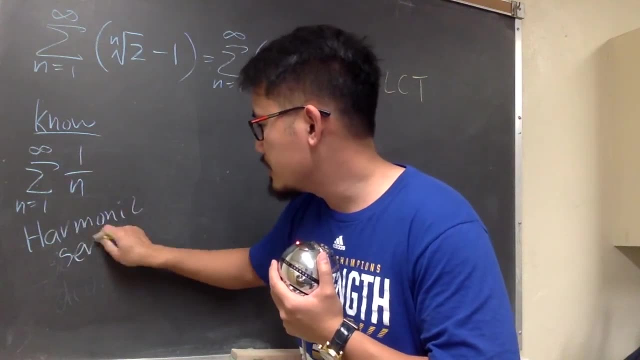 Just put down sigma where n goes from 1 to infinity, 1 over n. We know this is the harmonic series, so I will indicate that right here for you guys. Harmonic series, and we know it. It diverges, Okay. 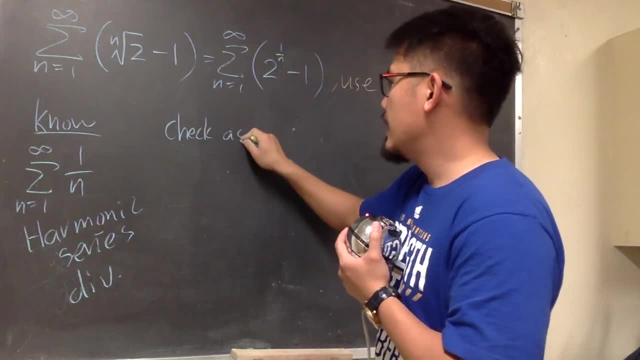 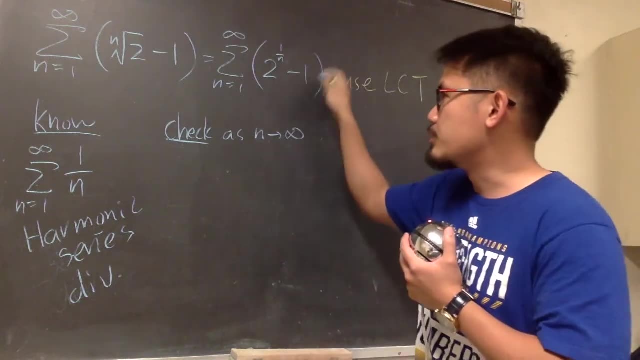 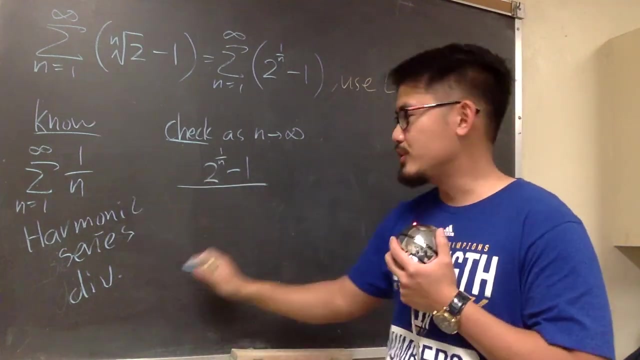 And now we will check the limit. We check as n goes to infinity, And let me just put this on the top and we will use this expression for now: 2 to the 1 over n minus 1, and then we divide it by the things that we know, which is the 1 over n. 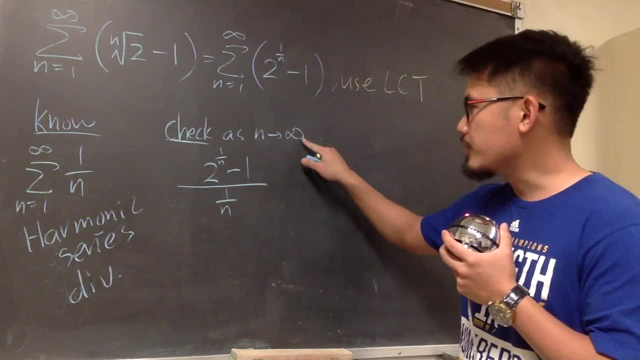 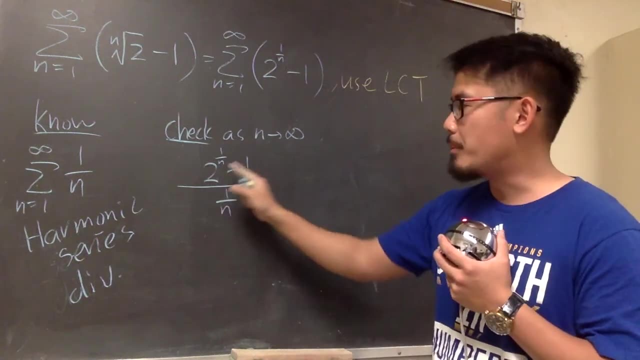 Alright. Here we have a small trouble When n is approaching infinity, 2 to the 1 over n, 1 over infinity, infinity is 0,. 2 to the 0 is 1, 1 minus 1 is 0 on the top. 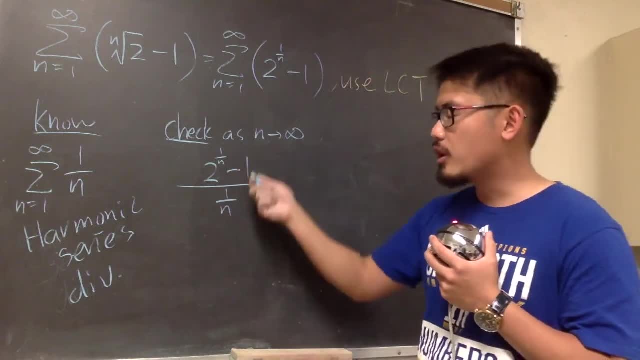 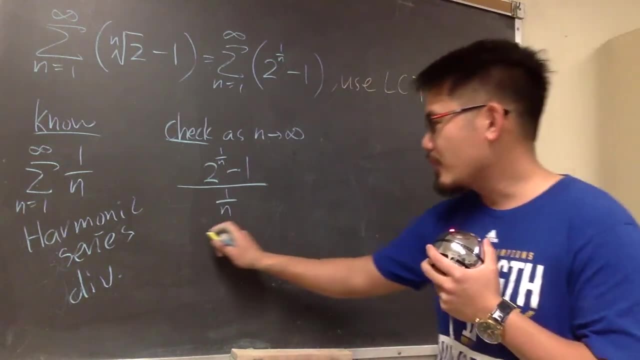 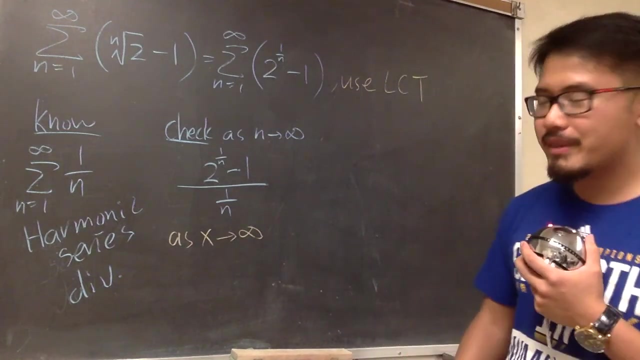 Infinity. here we get 1 over infinity, which is 0. This is a 0 over 0 situation. so we have to do more work, And the work that we will do is use Lafayette's rule. So I'm going to change that. this right here, in terms of x as x approaching infinity. 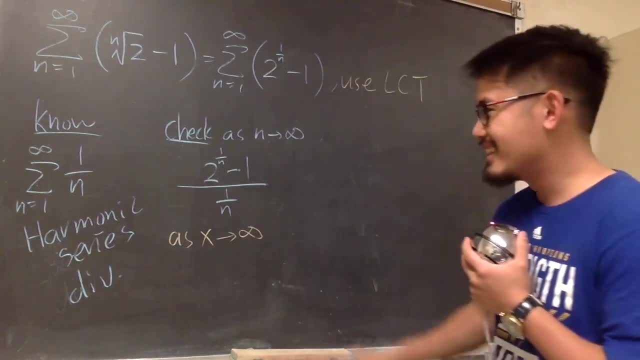 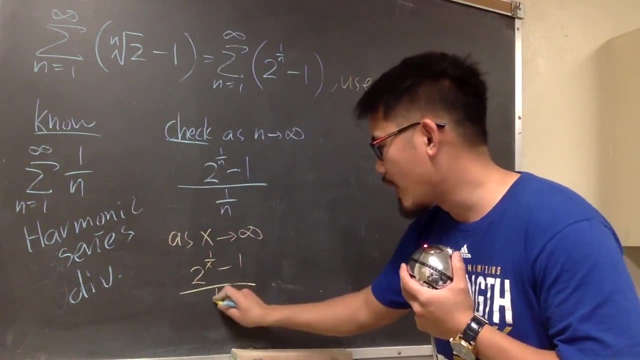 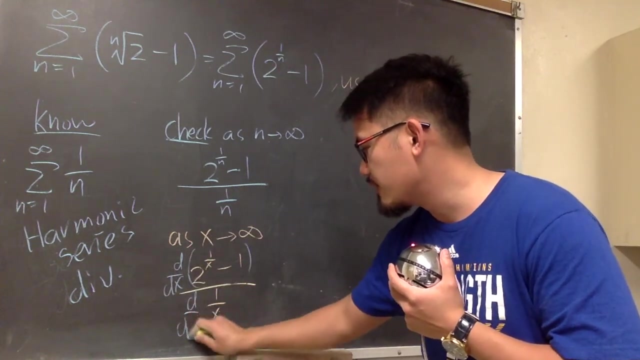 So I can be legitimate and take derivatives, Okay, Okay, So if we take the derivative of 2 to infinity, let's look at 2 to the 1 over x minus 1 over 1 over x, And we will just take the derivative on the top and then the derivative on the bottom to see what we get. 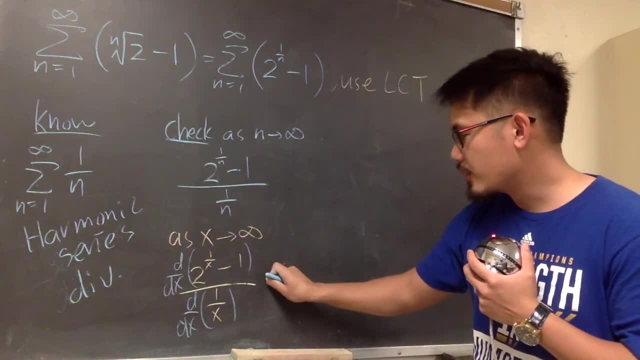 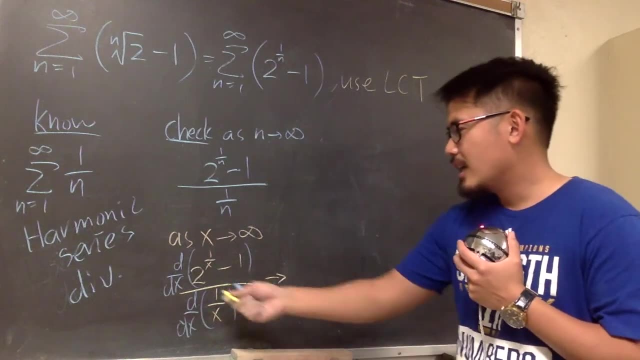 So if we do that, this is going to be well put down arrow. it's approaching because we're talking about limits. How can we take the derivative of 2 to something? I want to write this down right here for you guys. 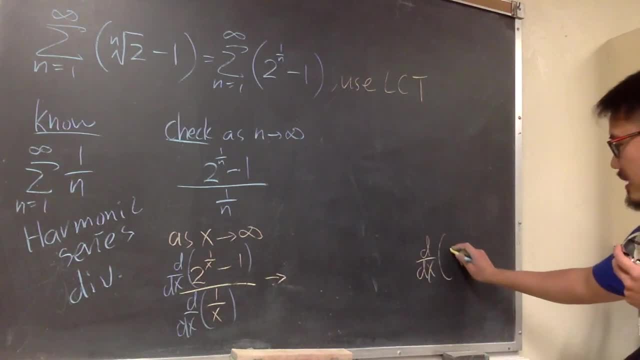 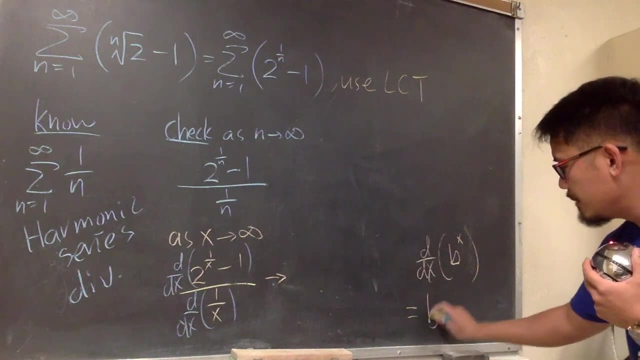 So recall that derivative of. let's say you have a base b to the x power. okay, This right here is the same, as we maintain the exponential form, which is b to the x, but then we multiply by ln, of whichever this value is ln b. 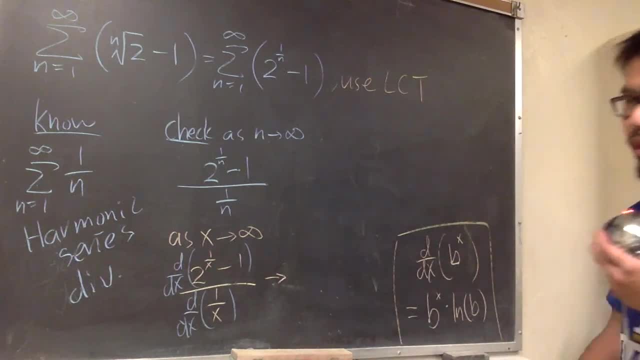 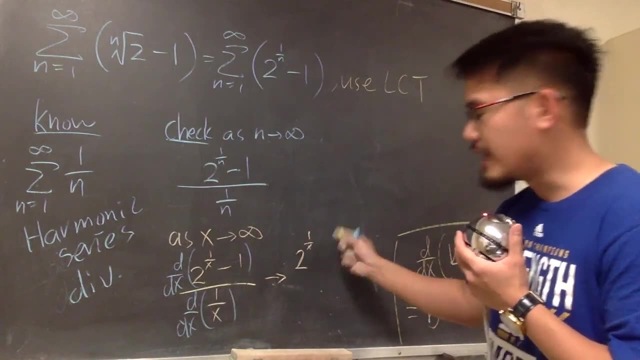 Okay. So this is the derivative formula that we are going to use. Anyways, 2 to the something, Okay, So 2 to the something, it first stays the same as 2 to the dot thing, And by this first. 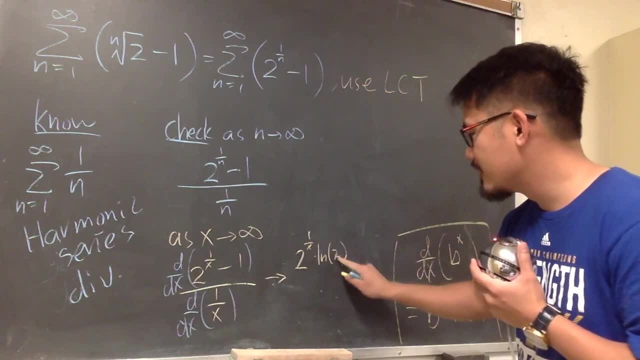 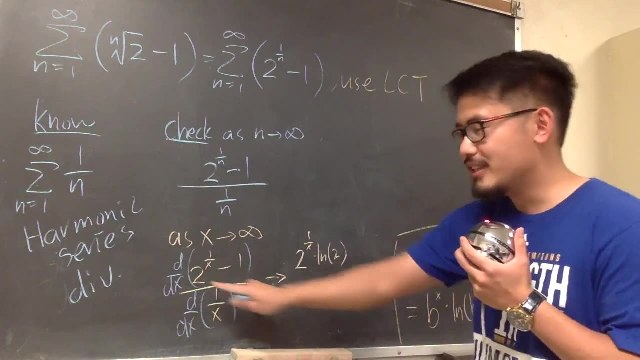 We first multiply by ln 2, okay, Once again 2 to the something it stays. but then this is a 2, it's not e, So we multiply by ln 2.. If it's an e, then we didn't have this okay. 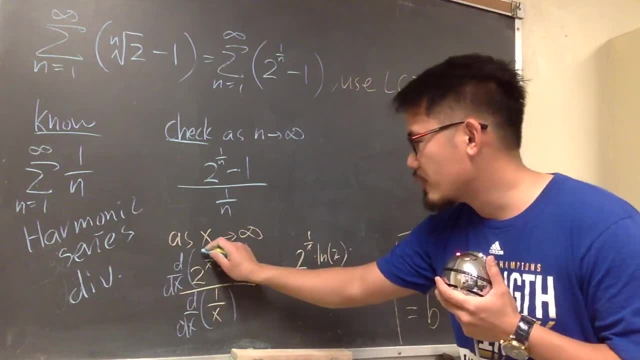 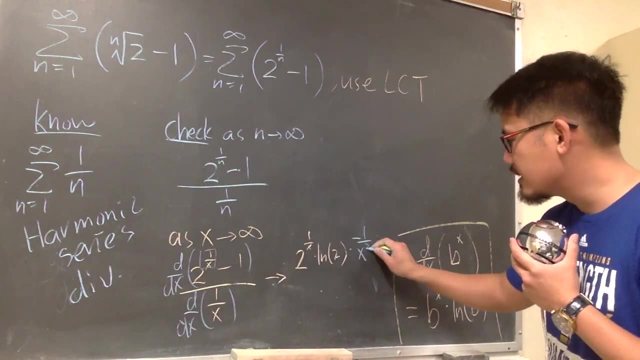 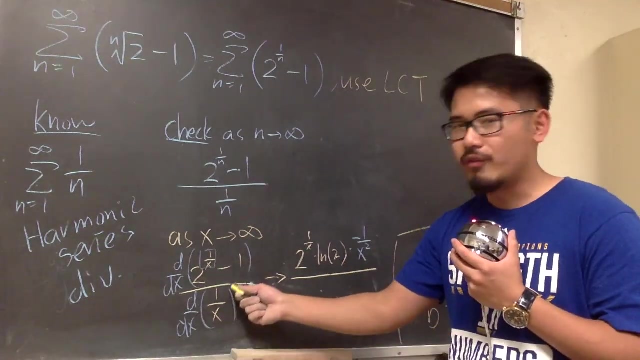 But then by the chain rule, we multiply by the derivative of that, And the derivative of 1 of x is negative. 1 over x squared, okay, And then we are going to divide it by the derivative of 1 of x. 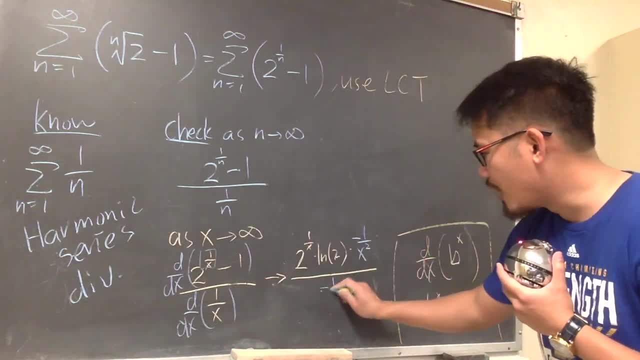 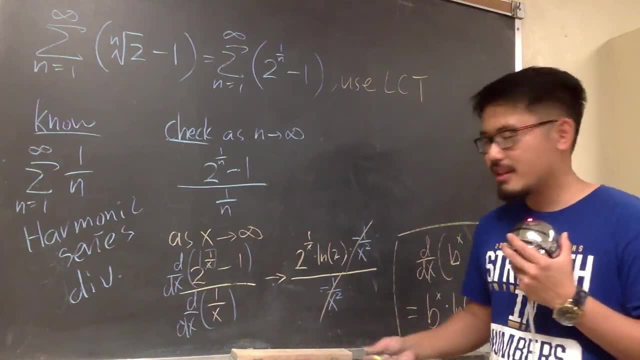 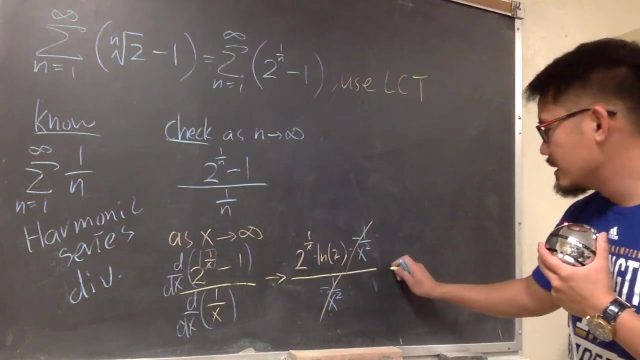 And once again, the derivative of 1 of x is negative, 1 over x squared, And you see that this and that cancel each other out completely, And let me erase this right here. Well, what do we get out of it? This is going to be approaching to, as x is approaching to, infinity. we have 2 to the 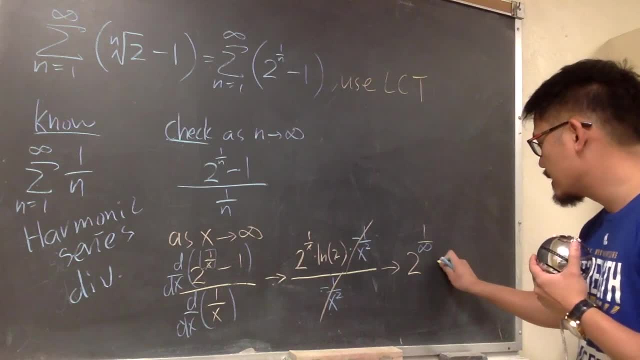 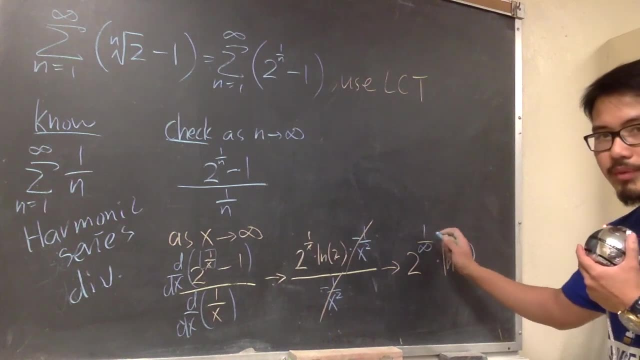 1 over infinity times, ln 2.. And then, once again, this is 0.. 2 to the 0's power is just 1.. So all this is pretty much approaching to just ln 2.. And this is the limit.